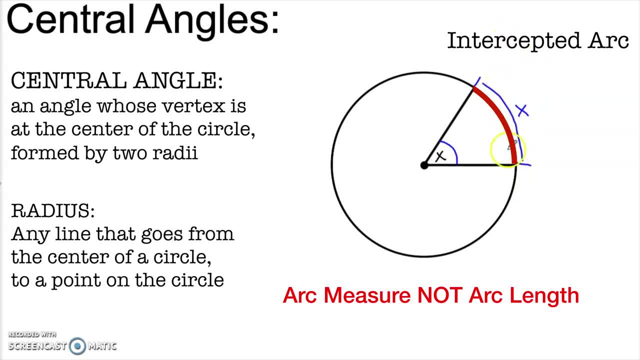 of the arc, not the length of the arc. The length would have to be measured in inches or centimeters or meters- some familiar unit like that. Since a full rotation is 360 degrees, it's useful to think about how much of the full rotation of the circle this intercepted arc is, And if we do that, a 40. 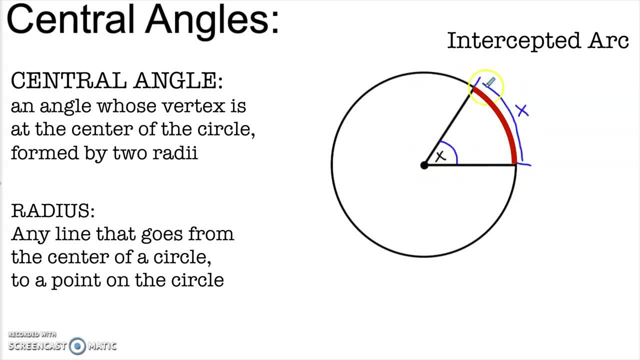 degree angle intercepts a 40 degree arc, A 90 degree angle intercepts a 90 degree arc, and so on. So a central angle is always equal to a 90 degree angle. So if I open this up to a 90 degree angle, 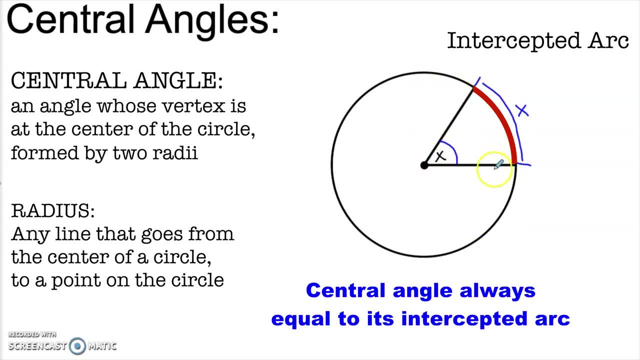 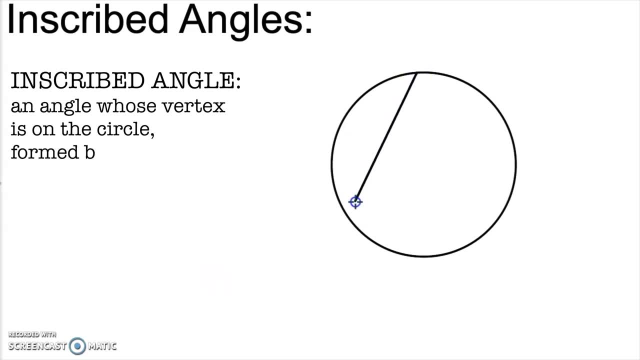 in measure to its intercepted arc. The next type of angle that we want to talk about is called an inscribed angle. An inscribed angle has a vertex on the circle itself and it's formed by two cords. A cord is just any line segment that connects two points on a circle. So if I pick two points on a 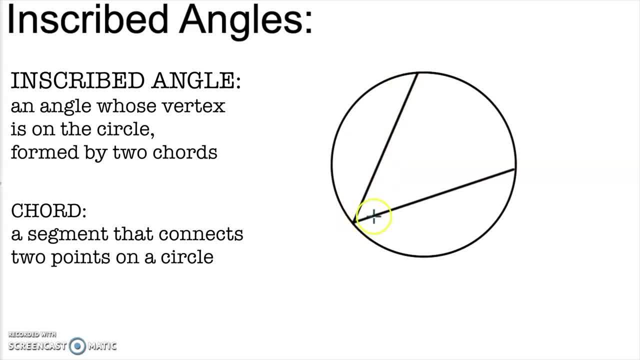 circle and connect those with a straight line. that's called a cord. So we have two cords here. they intersect on the circle itself. that makes this angle what we call an inscribed angle. Just like a central angle, an inscribed angle has an intercepted arc. If you imagine this angle biting down like a mouth, what part of the circle would 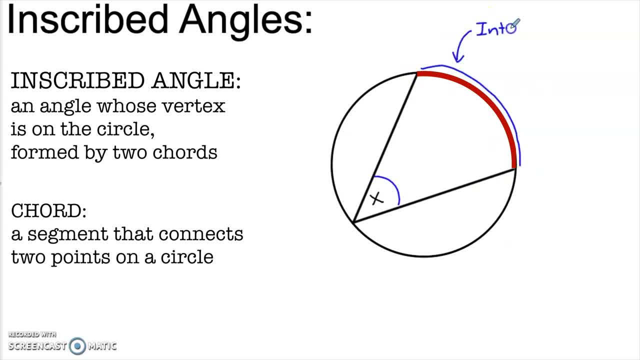 get chopped off, It would be this part right here, right? So we call that the intercepted arc. And for an inscribed angle there's this really interesting relationship where, whatever the angle is, that intercepted arc is always double. That is to say, if this angle has x degrees, then the measure of 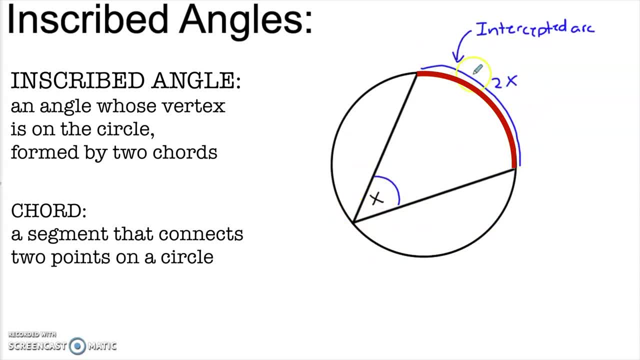 this intercepted arc is 2x. If the angle is 30, the arc is 60.. Notice that the center of the circle is not here, So it doesn't matter where the center of the circle is. It doesn't matter where the center of the circle is, as long as you have an angle formed by two cords and the vertex is on the. 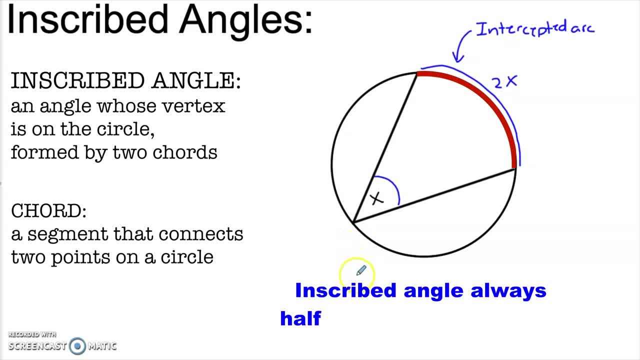 circle. it's going to be an inscribed angle and it will be half of its intercepted arc. Before I show you why that's the case, let me show you a few examples where we can use this relationship to figure out some variables in a circle. Here we have a circle whose center is O and we're being 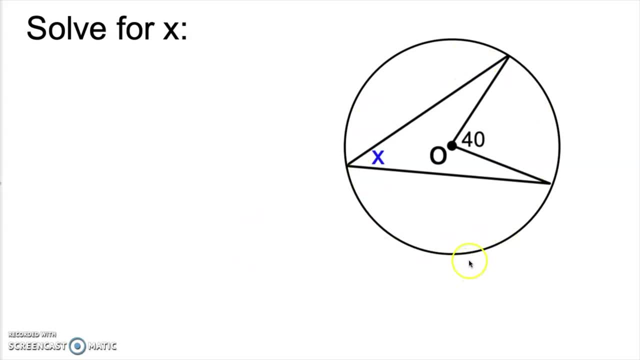 asked to solve for x. In mathematics we name circles by their center. So since this point is the center of the circle O- that's a pretty common choice for a circle- we would call this circle O. If the center was point A, we would call it circle A, And there's a few things going on in this circle. So x, the 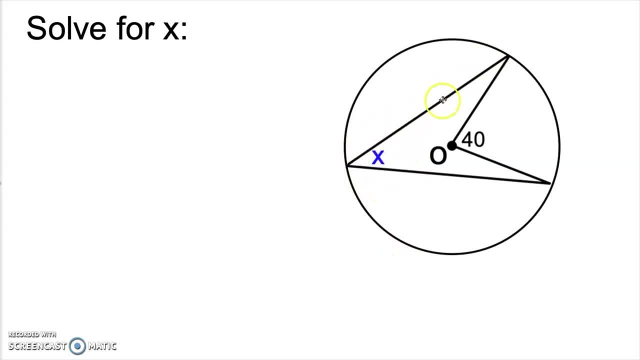 angle we're looking for is actually an inscribed angle. It's formed by these two cords, which means that it has to be half of its intercepted arc, or 2x in this case, But that still doesn't tell us what x is. But there's another angle in this circle, the 40 degree one. Notice that, that 40. 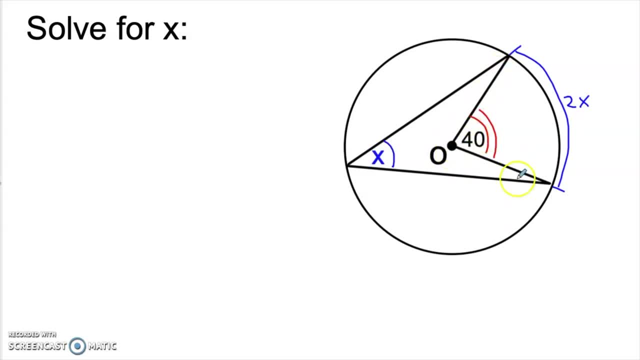 degree angle has a vertex at the center and is formed by two radii. That makes this a central angle, which means it is equal to its intercepted arc. But since it intercepted the center of the circle with its center m, one sign off our channel, So this represent the advantage of this angle. 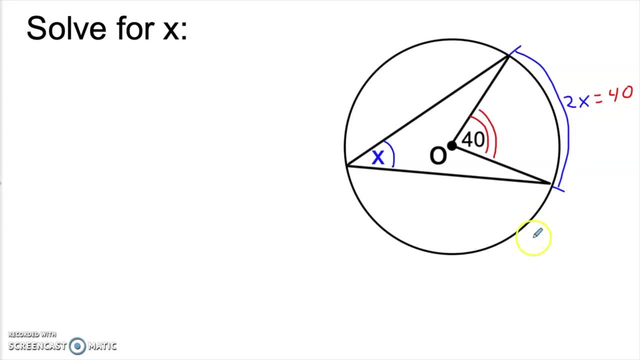 But since it intercepts the very same arc as the inscribed angle, that means that the arc has to be 40 degrees. Can u see that the intercepted arc is the same from both angles? If the 40lah angle were to close down like a mouth, it would bit off. exactly the same. 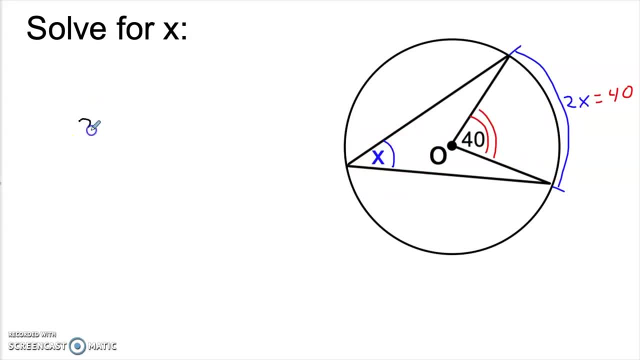 part of the circle, as the inscribed angle would if it were bite down like a mouth, Which tells us that 2x has to be 40. And, of course, if 2x is 40x is 20.. So there we have it. We solve for x by using both the properties of a central angle and an inscribed angle in the same circle. 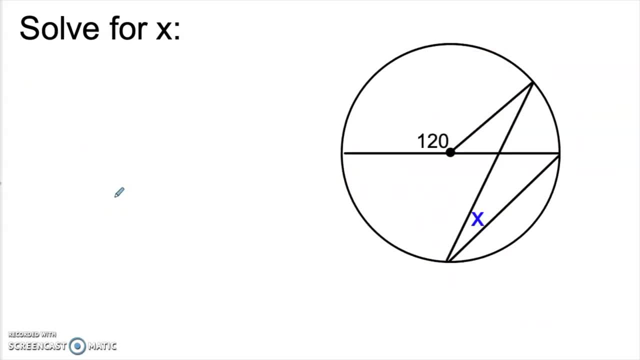 Here's another example where we have some central and inscribed angles. We also have a diameter in this circle right. This line goes straight across the circle and goes through the center. That means that it cuts the circle exactly in half. We're being asked to find this angle down here, which is an inscribed angle. 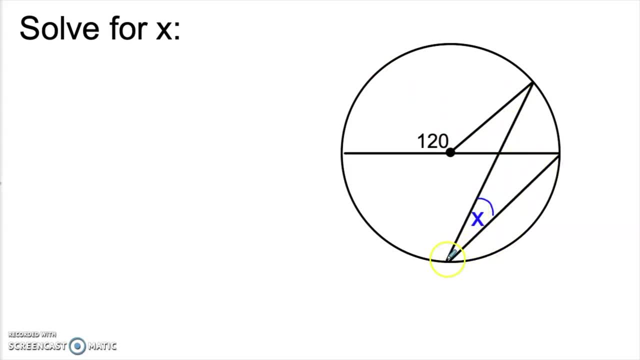 I know this because it's formed by these two chords and its vertex is on the circle. So let's first identify the intercepted arc. If we follow those two chords out and imagine that this angle bit down like a mouth, this is the portion of the circle that would get chomped off. 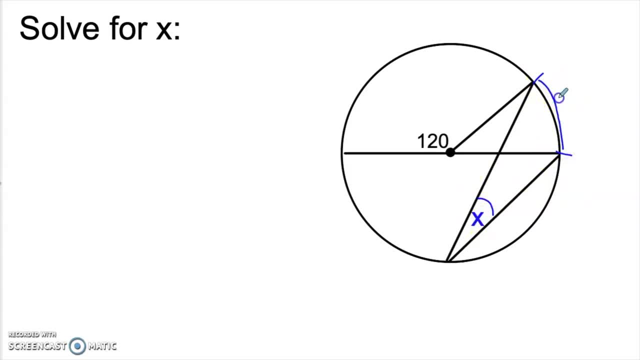 That means that this is the intercepted arc for this angle And since it's an inscribed angle, the intercepted arc has to be double. But how do we find out what x is? Well, if this angle is 120 degrees, having nothing to do with the circle, 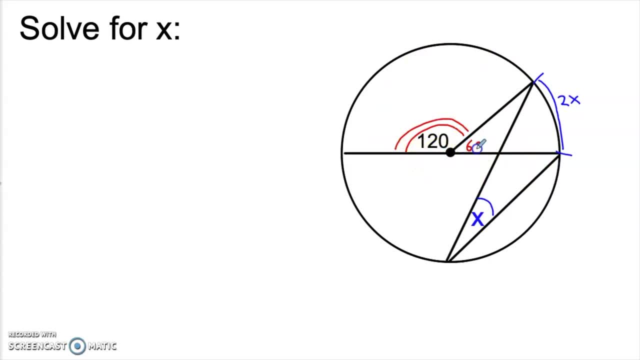 but just the fact that this is a straight line, doesn't that mean that this angle over here has to be 60 degrees? And isn't that 60 degree angle a central angle? It's formed by these two radii and it intercepts this very same arc. 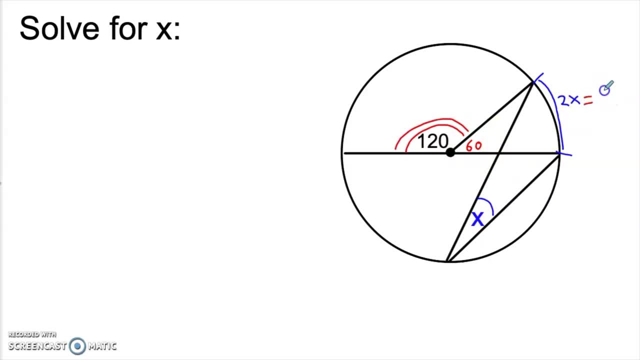 That means that if this central angle is 60, this intercepts this very same arc. This intercepted arc must also be 60. That tells us that 2x equals 60 and x equals 30.. One of the things I really like about circles is that there's often more than one way to solve a problem. 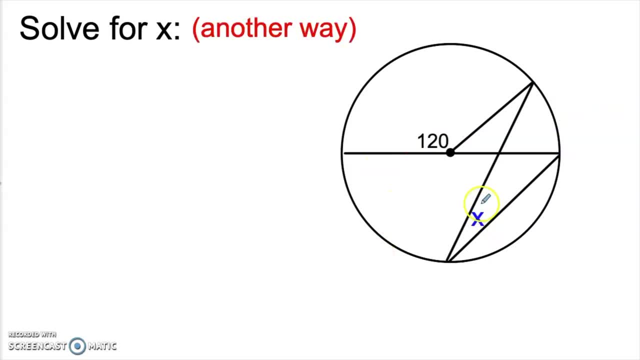 Let's take a look at this exact same problem, but let's solve it in a different way. So we start off looking for the same angle x. It's connected to this intercepted arc of the circle, which will have to be 2x. 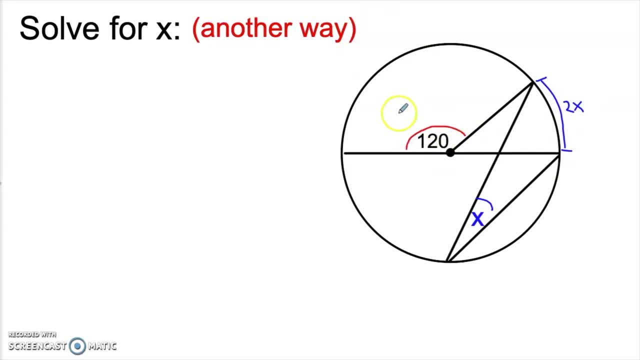 But this time let's notice that this 120 degree angle is itself a central angle. This is a radius, and this is a radius which means that this intercepted arc has to be equal in measure. so this big arc is 120 degrees. 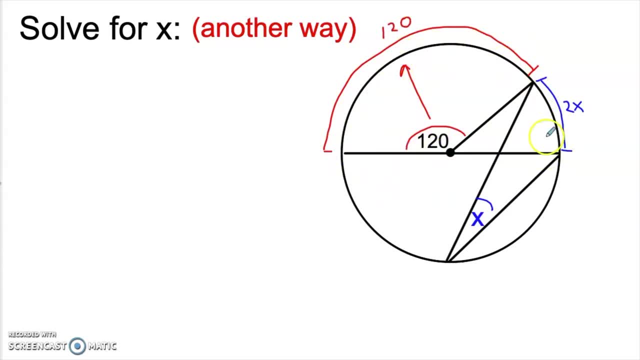 But wait a minute. since this is a diameter, it has to cut the circle exactly in half, which means that this top part, the blue and the red arc together, have to equal 180.. That tells us that 120 plus 2x has to equal 180, which means 2x equals 60, and again x equals 30. 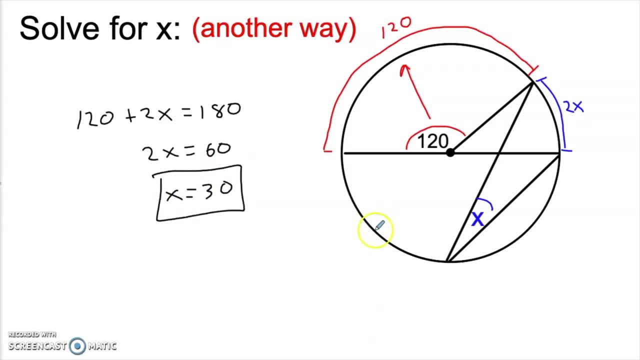 You see that Math always works. So there's the same problem two different ways. We get the same answer. of course, whether we solve it this way or this way, as long as we're using correct steps and making correct conclusions, we can solve a problem however we want to. 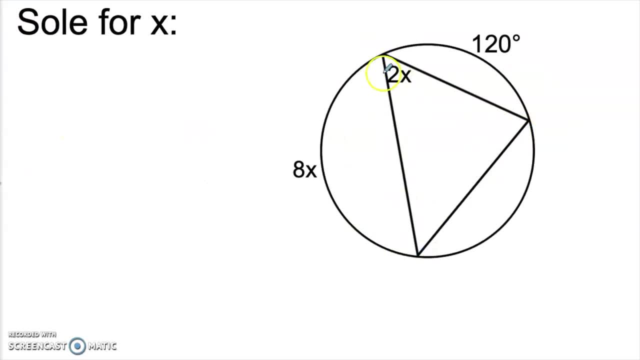 Let's take a look at another example. Here we have a triangle inside the circle, and this is actually called an inscribed triangle. for the same reason that these angles are called inscribed angles, They're set within the shape, So a polygon is said to be inscribed. 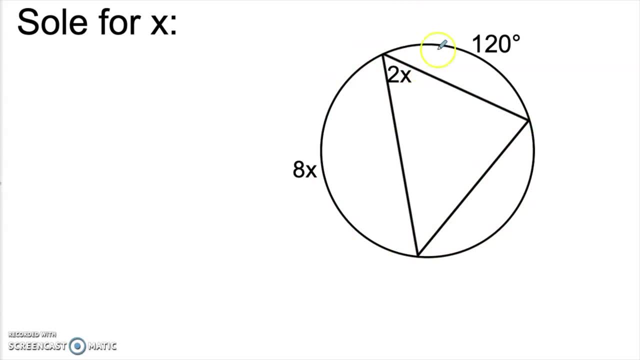 in a circle if all of the vertices of that polygon are on the circle. So here we have an inscribed triangle And if you notice, all three angles of this triangle are in fact inscribed angles. This one here that we're interested. 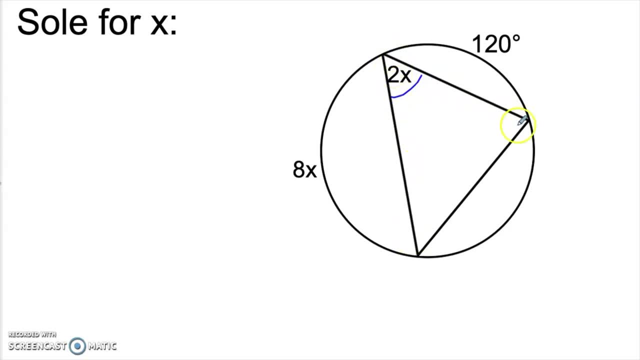 in that's labeled 2x is formed by these two chords, which means that its intercepted arc has to be double or 4x. Now how do we solve for x? Remember, if we go all the way around the circle, it'll be 360 degrees. 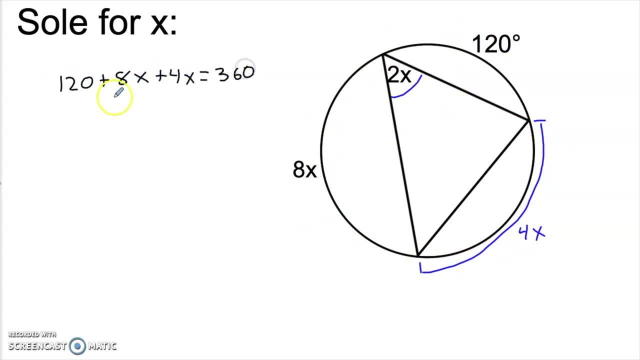 That tells us that 120 plus 8x plus 4x has to equal 360. So 12x is 240 and x is 20.. As we did with the last one, let's take a look at the same problem from a slightly different perspective. 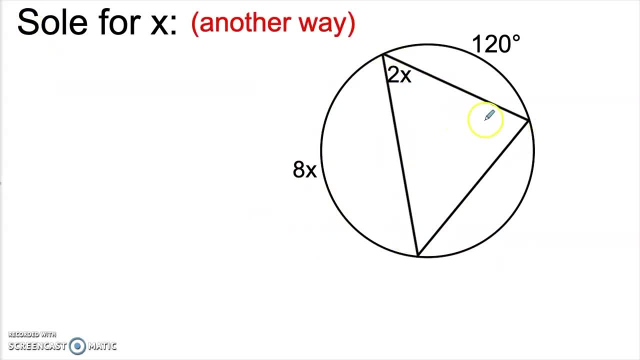 We know that this angle is 2x, but since it's inside of a triangle, if we could figure out the other two angles, we could then figure out what this angle is. So let's focus on those other two angles this time. 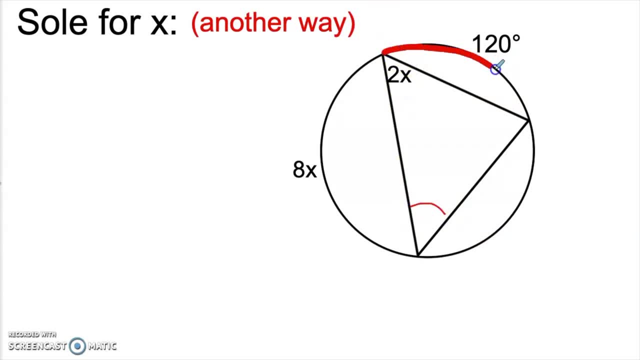 This angle here is an inscribed angle and this is the intercepted arc. Since an inscribed angle is always half of its intercepted arc, this angle has to be 60 degrees. What about this angle over here? Isn't this angle also formed by two chords and also an inscribed angle? 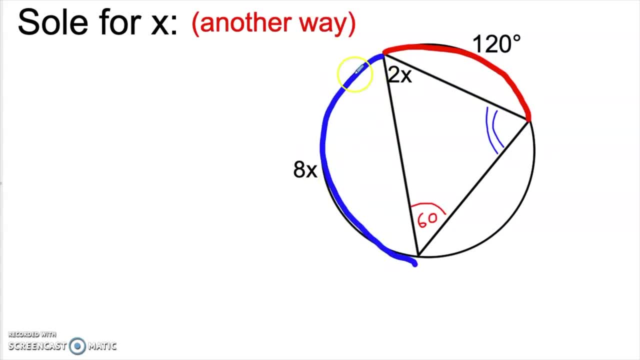 Its intercepted arc is over here. That means that if its intercepted arc is 8x, the angle itself has to be half of that or 4x. But now we can use the triangle to solve for x, Because we know that, like any triangle, the three angles have to add up to 180,. 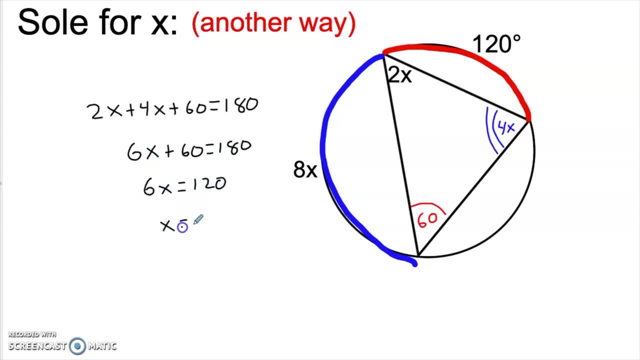 which tells us that 6x plus 60 is 180,, 6x is 120, and x is 20.. So there you go. Once again, we have the same problem, same result: x is 20 both times. 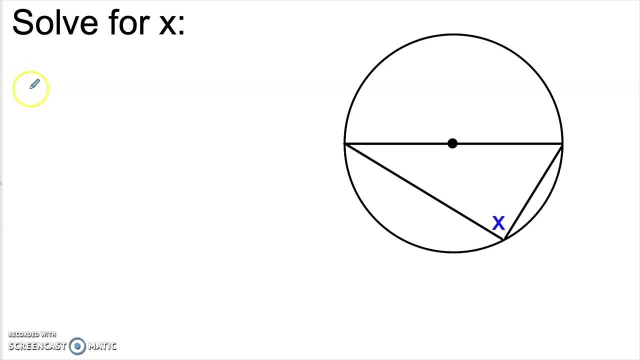 but a different method. One last example before I show you why inscribed angles are half of their intercepted arc. this is a really interesting one. Here we have an inscribed angle and you can see its intercepted arc. is this whole piece of the circle here? 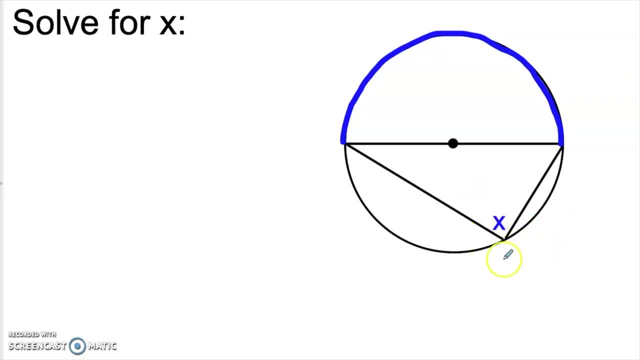 And at first you might think, hey, wait a minute, we don't have enough information to tell what x is Because there are no other numbers in this picture. But wait, this is a diameter. I know that because it goes through the center of the circle. 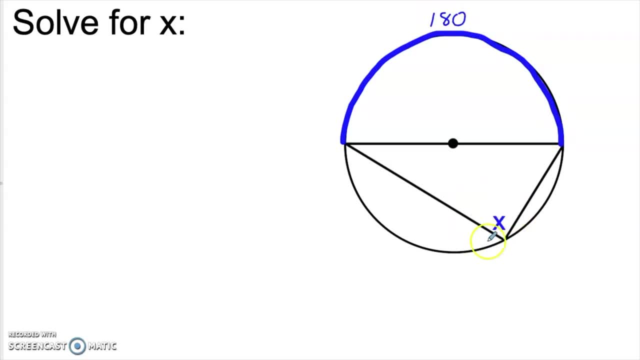 So that's a 180 degree arc there, But this is an inscribed angle. It is formed by two chords that intercept this 180 degree arc. So what type of an angle is this? That has to be a right angle, So in this case, x is 90.. 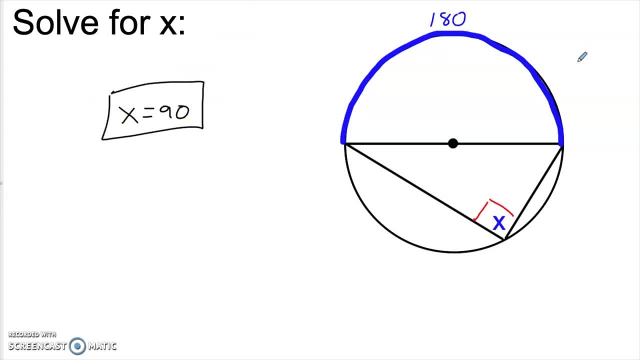 But that's actually leaving out something that's pretty amazing about what's going on right here. Take a look at this. Here I have a circle with a diameter and an inscribed angle so that the two chords intercept the entire half of the circle as I move this vertex around. 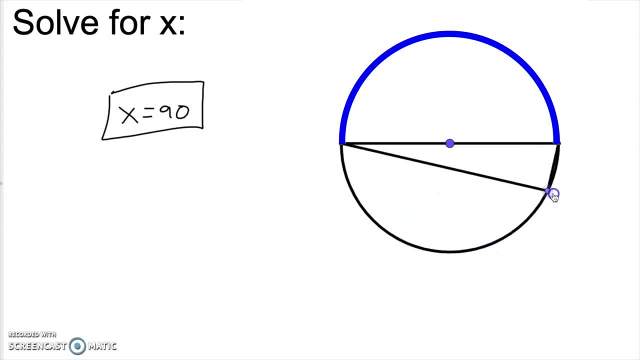 What do you notice about the size of that angle? Can you see that it's always a perfect right angle? It cannot be anything else because the inscribed angle is always half of its intercepted arc. It doesn't even matter if I bring it up to the top of the circle. 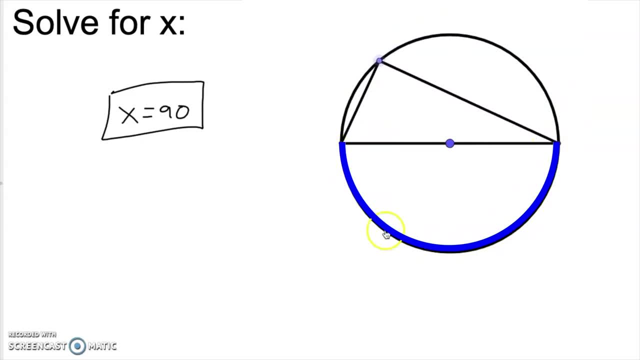 It's still going to be a right angle because now it intercepts the bottom half of the circle. So any angle inscribed to a semicircle is always going to be a right angle. Pretty neat, right? But of course that relies on this idea. 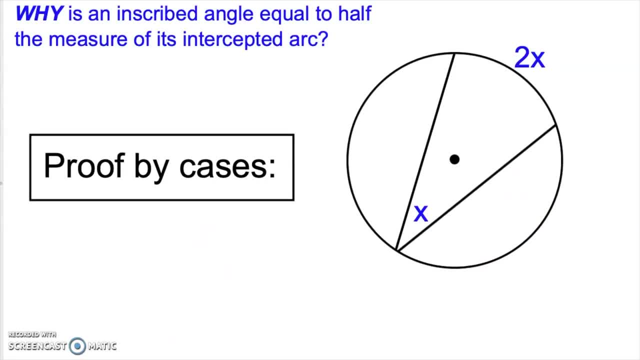 that the inscribed angle is always half of its intercepted arc. So why is it that the inscribed angle is always half of its intercepted arc? This is actually a lovely bit of mathematics for high school geometry, because we do something called proof by cases in order to demonstrate this. 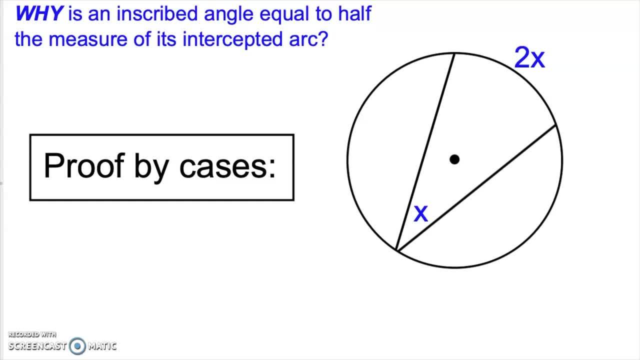 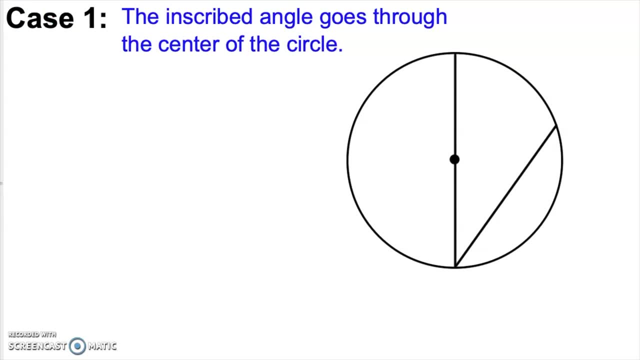 relationship Proof by cases means that we can make an argument that explains why it works, but only for certain times. We have to make a different argument for other times. The first is when we have an inscribed angle that goes through the center of the circle. We'll call this case one. 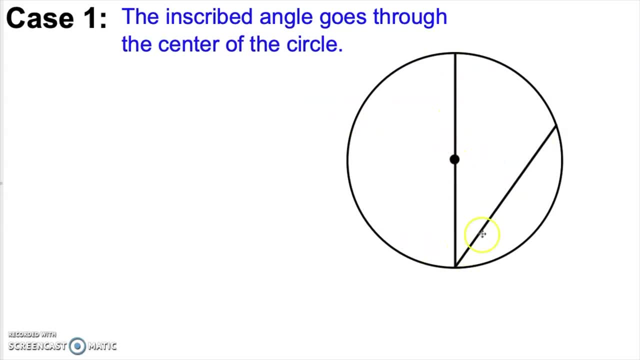 So here we have an inscribed angle. There's the center of the circle And, of course, these are two chords. Notice that this one is a diameter, So let's go ahead and label this inscribed angle X. Our goal is going to be to demonstrate that this intercepted arc is 2X. 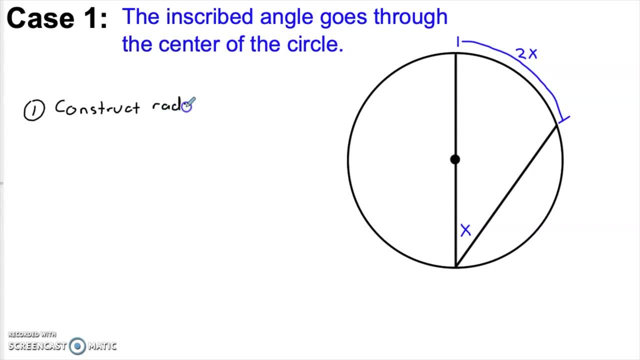 In order to show why this is true, I'm going to need to construct a radius. Of course, there are many radii I could place into the circle, But the one that I want to construct is this one right here, from the center of the circle to this one end of the inscribed. 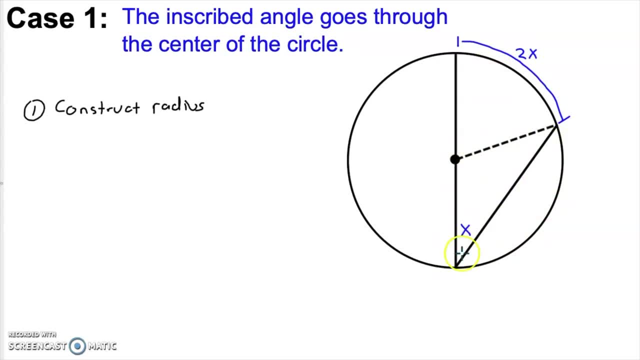 angle. Once I do that, notice that we get a triangle where the inscribed angle is one of the angles of that triangle. But it's not just any triangle. Since this is a radius, it has to be the same length as any other radius in the picture. 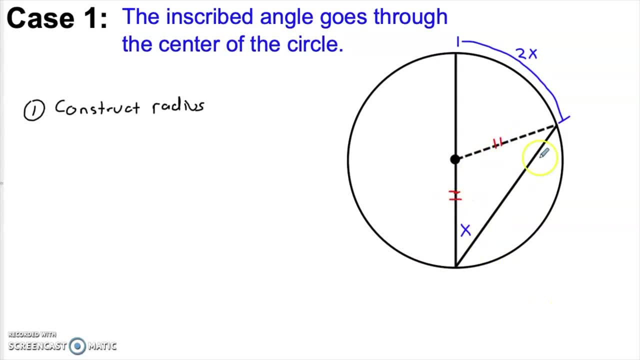 Specifically, I'm interested in the fact that it's the same as this radius. That means that this is not just any triangle, It's an isosceles triangle And this angle, our inscribed angle, is the same as this angle here. 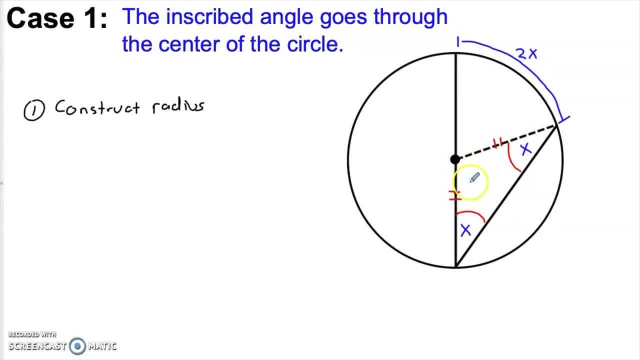 So this is also going to be X. I don't know what this third angle is, but that's OK. Instead, I'd like you to focus on this central angle. This central angle is equal to its intercepted arc. Now, remember, we don't actually know. this is 2X. 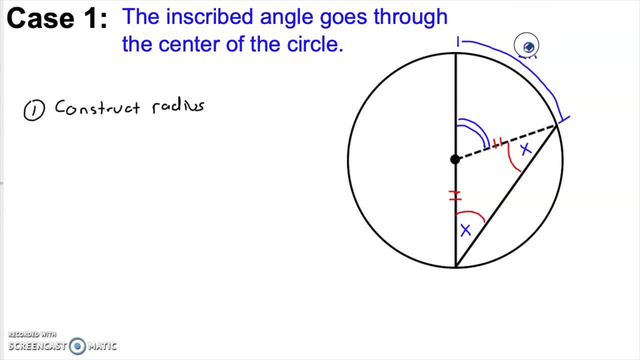 We're trying to prove that that's the case, So let me actually just go ahead and erase that, just so we don't confuse ourselves. This central angle has to be the same as this intercepted arc here, And I would like those to both be 2X. 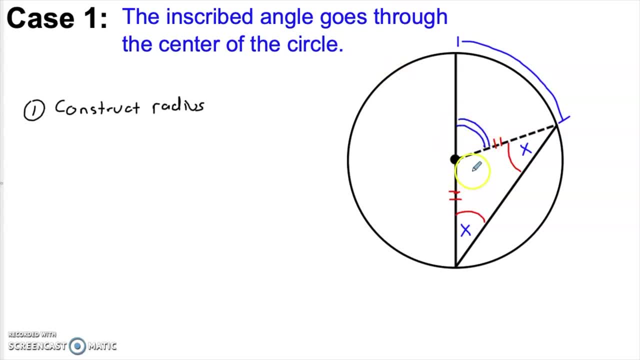 But how do I know they are? Well, this angle is not just a central angle, It is also an exterior angle to this triangle. Remember how an exterior angle works. If you have a triangle and you extend one of the sides, that exterior angle is always equal to the sum of the non-adjacent interior angles. 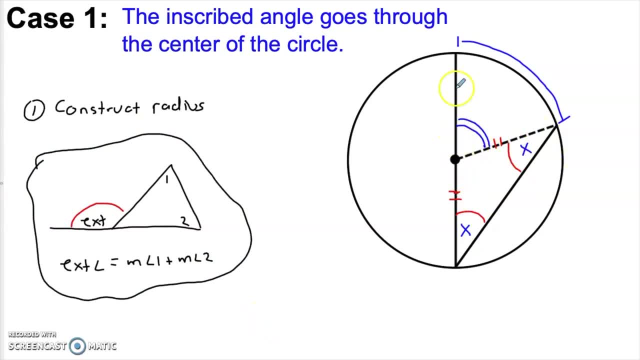 So in this triangle, this angle is formed by extending this side of the triangle, which means it's an exterior angle and it is equal to the sum of the non-adjacent interior angles. In other words, this central angle has to be 2X. 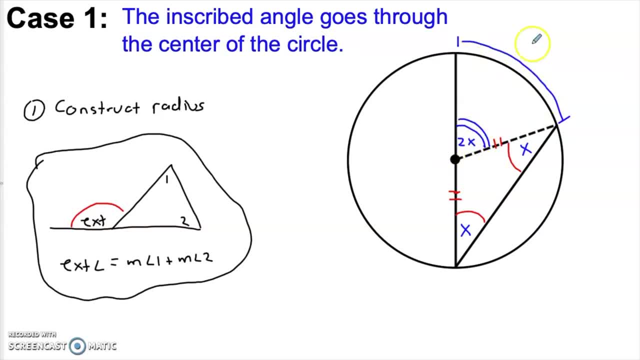 But if this central angle is 2X, then its intercepted arc is 2X, And there you have it. The inscribed angle that we started with down here is exactly one half of its intercepted arc. Boom, Done right. Well, not so bad. 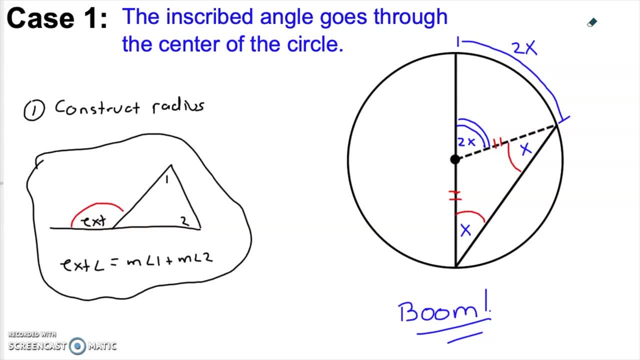 Let's go fast. This feels very satisfying and it is completely convincing, But this is only case one. Why aren't we done here? Well, there was a pretty big assumption we made in the beginning. Do you remember what it was? This inscribed angle goes right through the center of the circle. 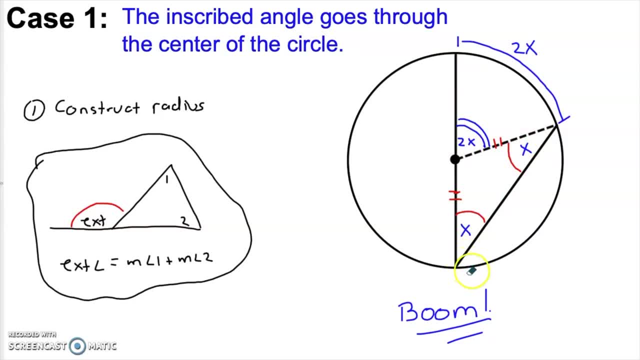 In other words, one of the chords was a diameter. That's not always the case, And if we change that fact, then this argument falls apart. So that's why this is a proof by cases. Let's take a look at case two. 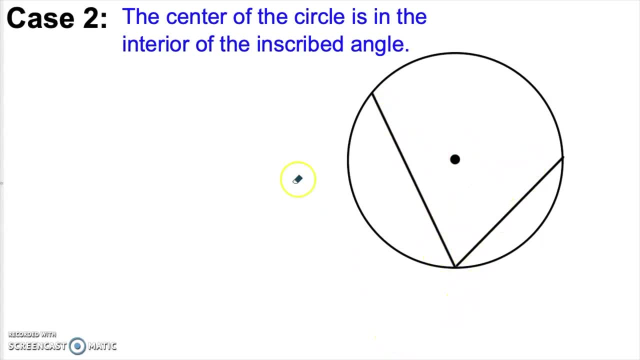 What if the center of the circle is somewhere on the inside of our inscribed angle? In my class I talk a lot about problem solving techniques. If you can reduce a problem that you don't know how to solve into a problem that you already know how to solve, then you're done. 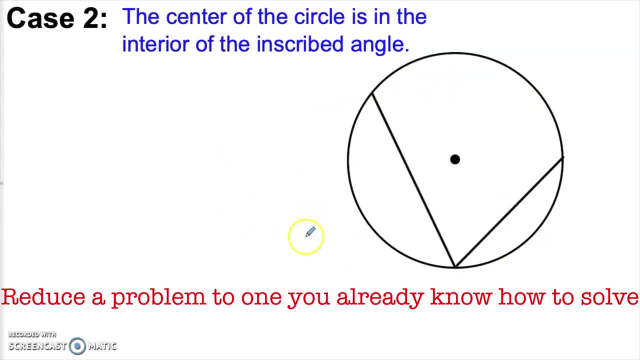 And we can actually do that here by just adding one line to this picture. Remember, if our inscribed angle goes through the center, we already know how to solve that. That was case one, So let's go ahead and construct a diameter. 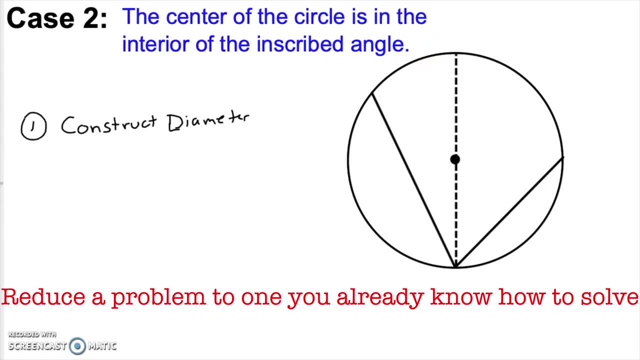 Again, I'll do that with a dotted line to remind us that it wasn't there to begin with. And now we have to be a little bit careful, because the original angle that we were talking about is that This entire angle, which has now been split into two angles. 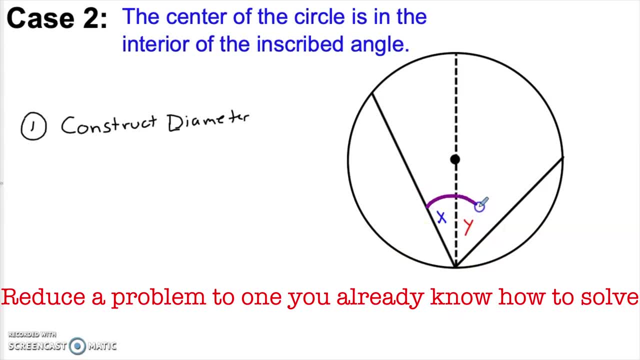 let's call them X and Y, and I'll go ahead and mark the original angle, our inscribed angle, in purple. What we'd like to be able to show is that the original angle, which is X plus Y, is one half of its. 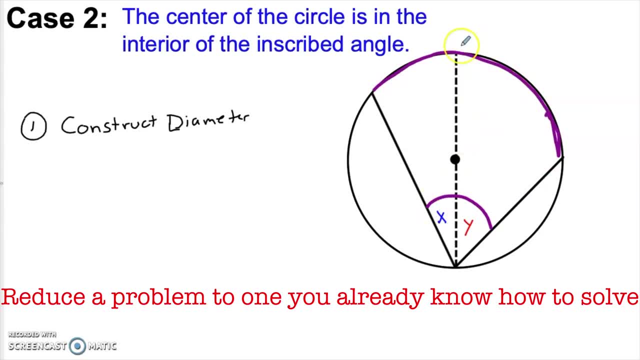 intercepted arc, this great big purple arc here. But do you see what happened when we put that diameter in Something kind of magical? Instead of one inscribed angle, now we have two inscribed angles, right Aren't, X and Y, both inscribed angles. 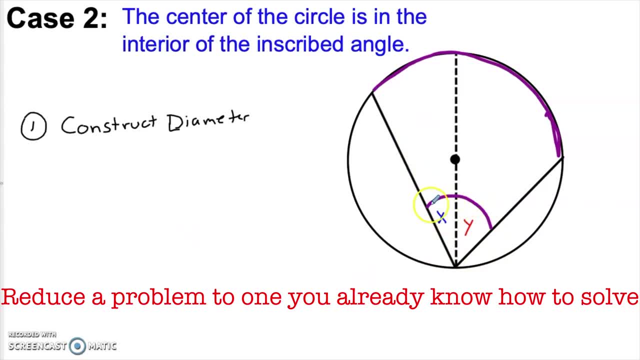 And not only that, they're both case one angles X is an inscribed angle that goes through the diameter, and Y is an inscribed angle that goes through the diameter, which means that we've already proven that this angle X intercepts an arc that is exactly two X and this angle Y. 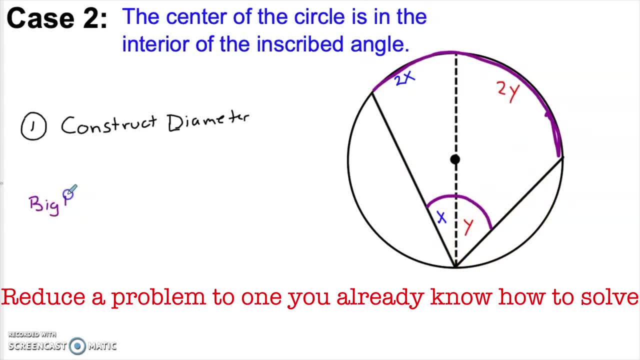 intercepts an arc that is exactly two Y. That means that the big purple arc is two X plus two Y, which of course is the same as two times X plus Y. But wait a minute. The original inscribed angle is X plus Y, which is exactly half of the big purple. 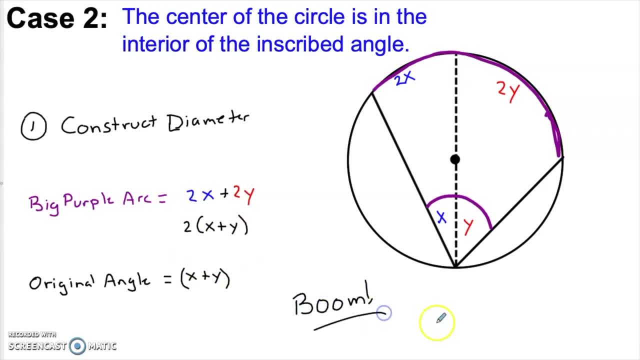 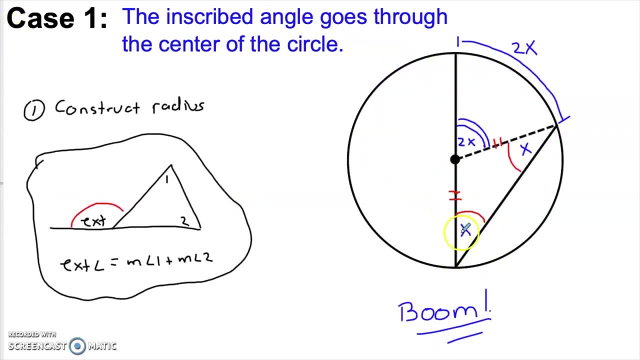 arc. So there you have it Inscribed. angles are always one half the intercepted arc, Or is it? Well, we know that if the angle goes through the center of the circle, we can prove it with this argument, case one: We know that if the angle goes around the center of the circle, 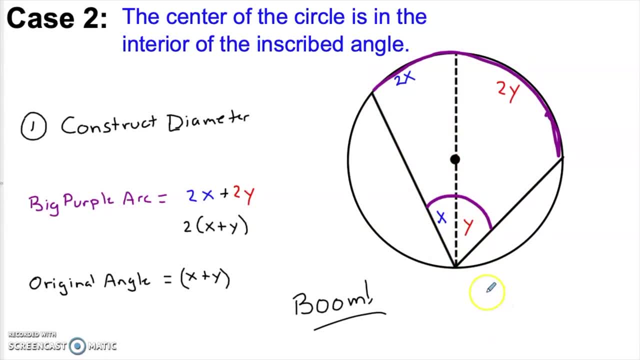 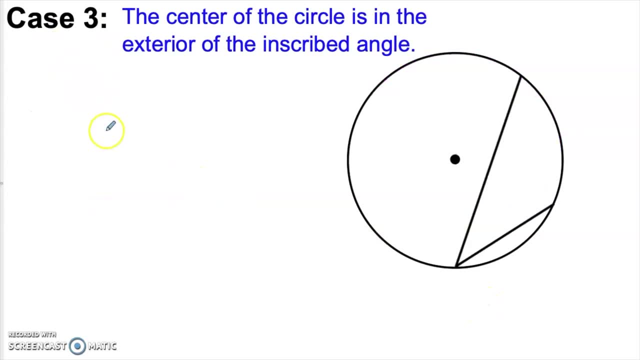 we can prove it with this argument. case two. But there is still one more case we haven't considered. Can you think of what it is? What if the inscribed angle is set up so that the center of the circle is outside of the angle? Again, we're interested in this angle right here. 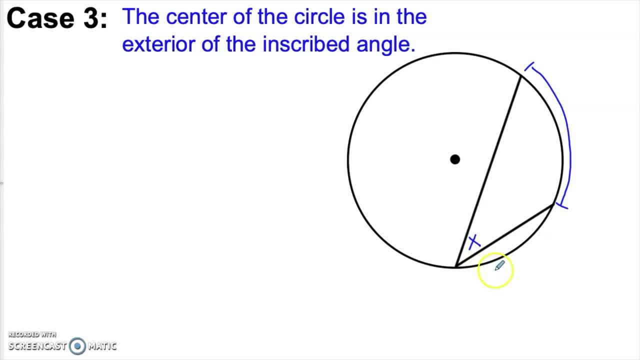 This is the inscribed angle, So we're going to take the intercepted arc that intercepts this arc. What we'd like to be able to show is that this arc has to be two, X or a double the inscribed angle. The way that we're going to do that is by, once again, 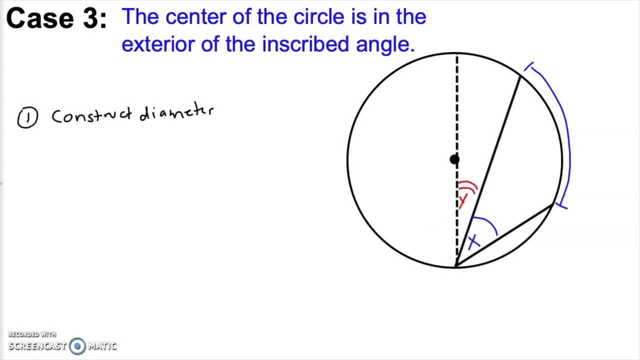 adding in a diameter, I've now created some case one angles. This angle right here, let's call it Y, is an inscribed angle. That's a case one angle Goes right through the center of the circle, which means that we know that its intercepted arc has to be two Y. 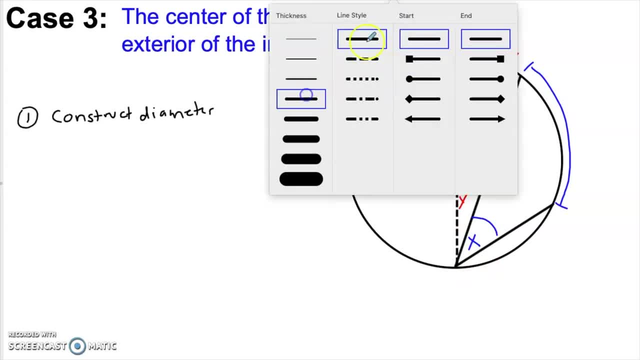 And here's the tricky part: This large angle, all the way from there to there, is also an inscribed angle. It's formed by this chord and this diameter, So that angle has to be one half of its intercepted arc, because that's also a case one angle, But it has this great big intercepted arc. 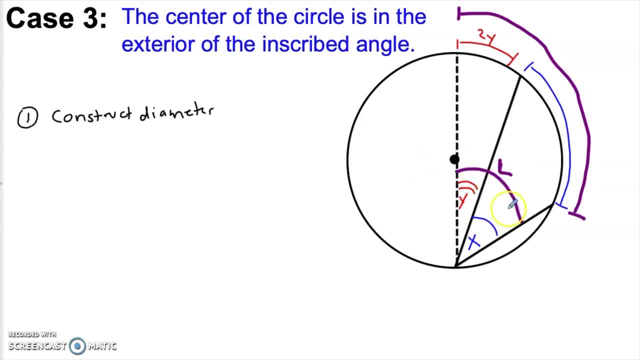 Since this is such a large angle, let's go ahead and call it L for large. Since it's an inscribed angle, its big intercepted arc is double 2L. Now let's go ahead and collect what we have here in an equation. 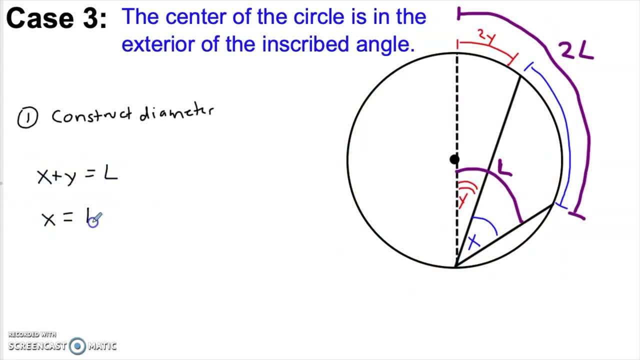 We know that X plus Y has to equal L, and that means that X is equal to L minus Y. Remember, this is our original inscribed angle. Let's do the same thing with the big arcs. It's also true that 2Y plus the blue arc is equal to 2L, that great big arc. 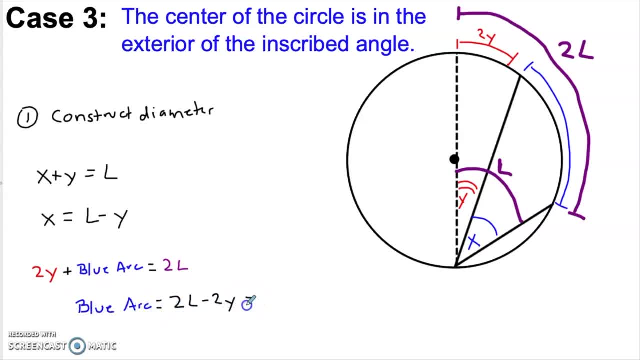 But that means that the blue arc is 2L minus 2Y, which is 2 times L minus Y. And there you see that. And now we can see that X minus L Y, the original inscribed angle is half of 2 times L minus Y. 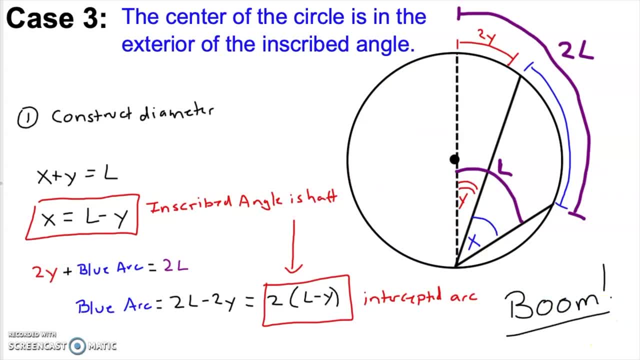 The intercepted arc. Boom, That time we've got it. All three cases together cover every possible inscribed angle we could have, So I'm going to go ahead and put a proof box there for those of you in the know. That's going to do it for this video.